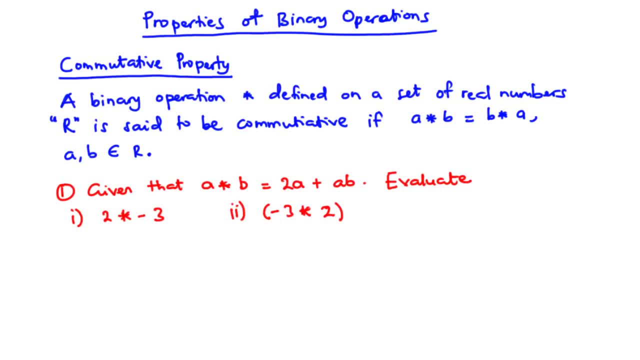 R is said to be commutative if A star B is equal to B star A, where A and B are all members of the set R. Now we have a question here. Given that A star B is equal to 2A plus AB, we are going to evaluate I, 2 star negative 3 and then I. I. 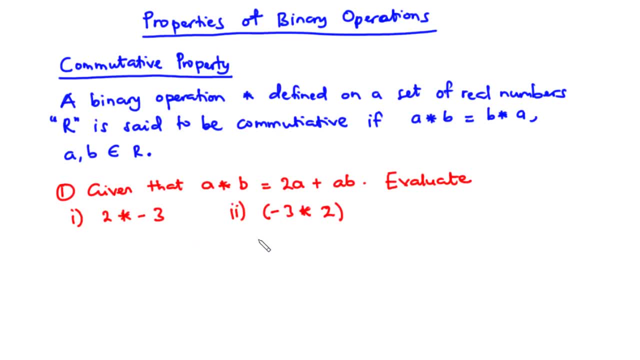 negative 3 star 2.. So let's solve this problem Starting from I: 2 star negative 3.. Now we are going to use this rule, the rule for the binary operation A star B, So our A is going to be 2 and then our B is going to be negative 3.. So we are going to substitute 2 and negative. 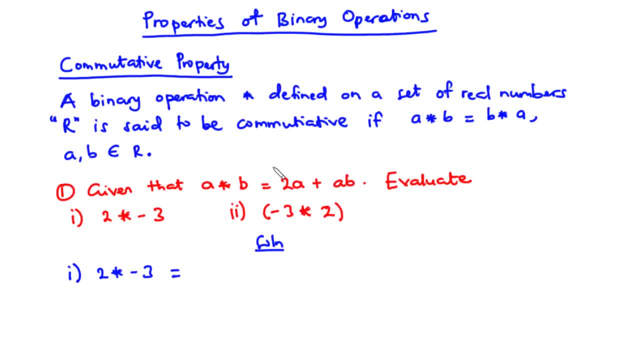 3 in place of A and B in this binary operation. So we have 2 star negative. 3 equals 2 times 2 plus 2 times negative 3.. 2 times 2 is 4.. 2 times negative 3 is negative 6. So we have: 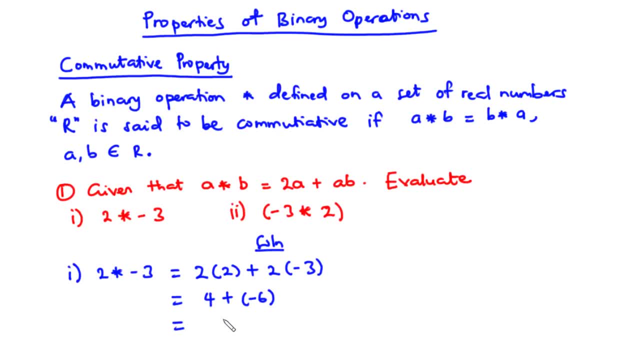 4 plus negative 6 is negative 2.. Now let's solve for II, that is negative 3, star 2.. We are going to apply the same rule, 2A plus AB, to this binary operation. So our A is negative 3 and then this time our B is 2.. So we have 2 times negative 3. 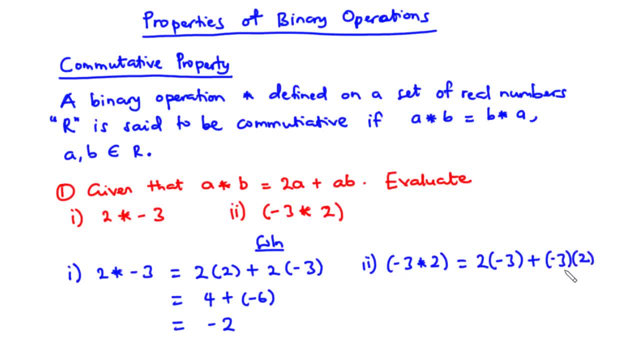 negative 3 times 2.. 2 times negative: 3 is negative, 6. Negative 3 times: 2 is negative, 6. So negative 6 minus 6 is negative, 12. So negative 3 star: 2 is negative 12 and then 2 star negative 3. 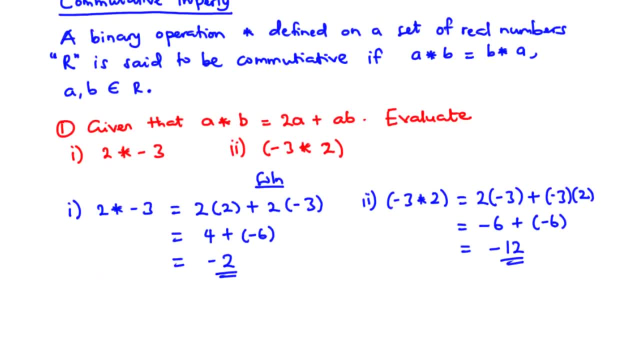 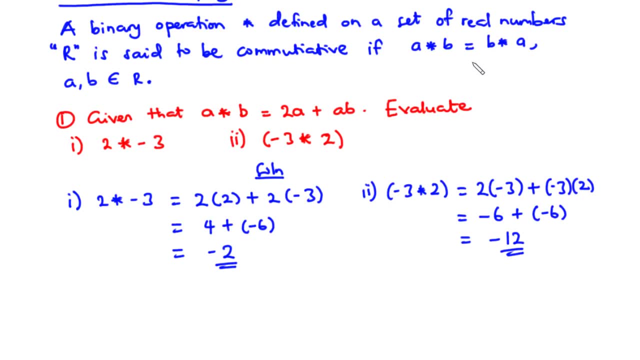 is negative 2.. Now we said earlier that for a binary operation to be commutative, then a star b should be equal to b star a. Notice here that 2 star negative 3 is negative 2, and then negative 3 star 2 is negative 12.. So since 2 star negative 3 is not equal to negative 3, 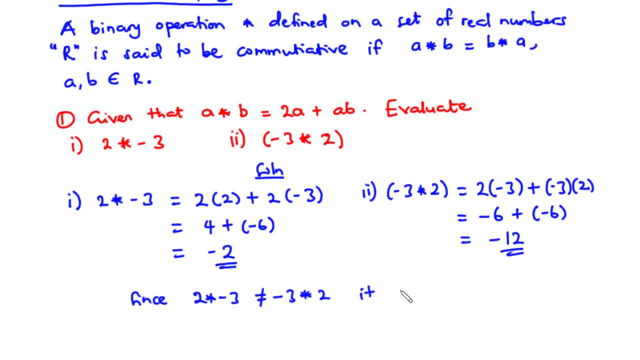 negative 3 is negative 3.. So we can say that 2 star negative 3 is negative 2. Star 2. It follows that the binary operation star is not commutative. So that was a very simple one. So for us, 2 star negative 3 is not equal to negative 3 star 2.. 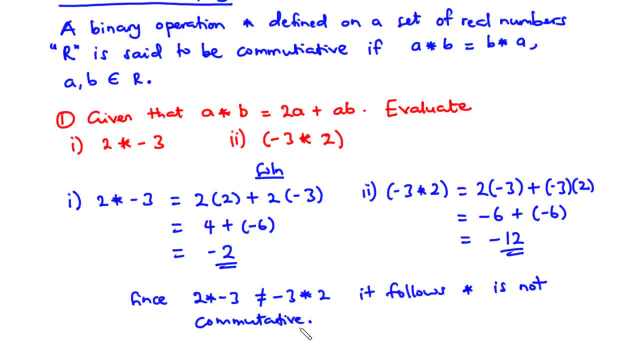 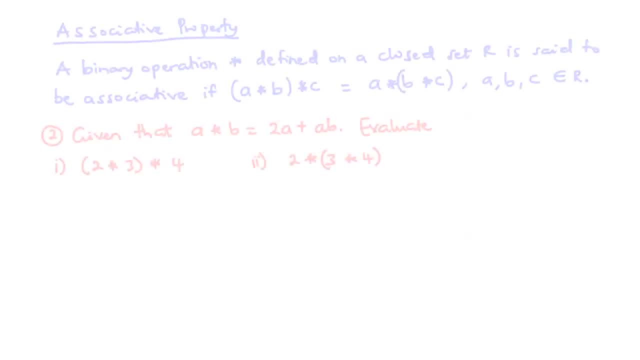 It follows that the binary operation star is not commutative. Now let's move on to the next property, the associative property. So for the associative property we say that a binary operation star defined on a closed set R is said to be associative if a star b in a bracket star c is equal to a star into bracket b, star c. 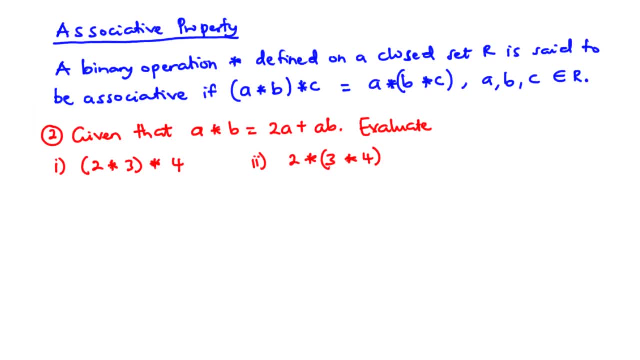 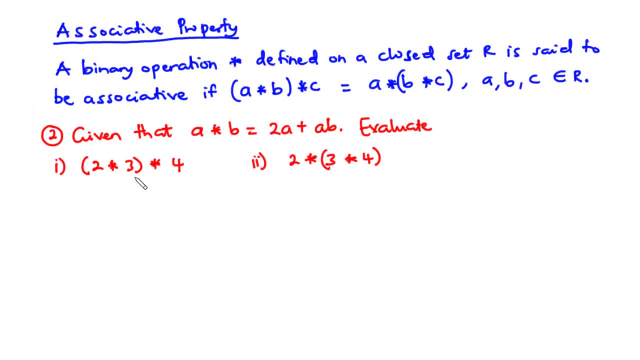 We have a question we want to answer. We have a question we want to answer. We have a question we want to answer. We want to validate whether 2 star 3 in a bracket star 4 is equal to 2 star into bracket 3, star 4?. 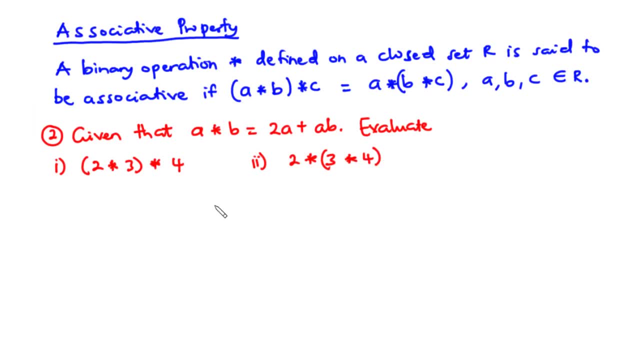 So we are going to evaluate the two and then compare. If they are the same, we conclude that the binary operation star is associative. If they are not the same, then the binary operations star. it's not associative. So let's start off with a. 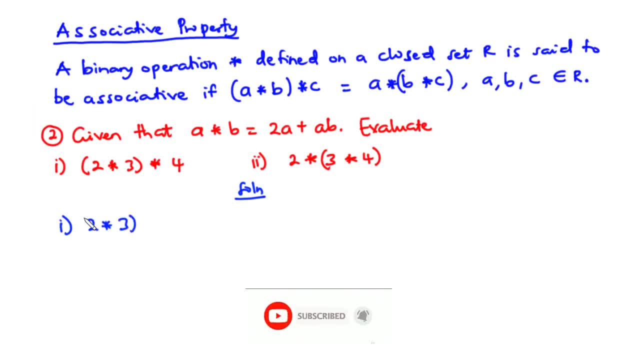 2 star 3 in the bracket star 4. so first of all we are going to use the binary operation to combine 2 and 3. afterwards we are going to combine the results of 2 and 3 and then 4. so we are going to use a star b, so our a is 2, our b is 3, so that's going to be 2 times. 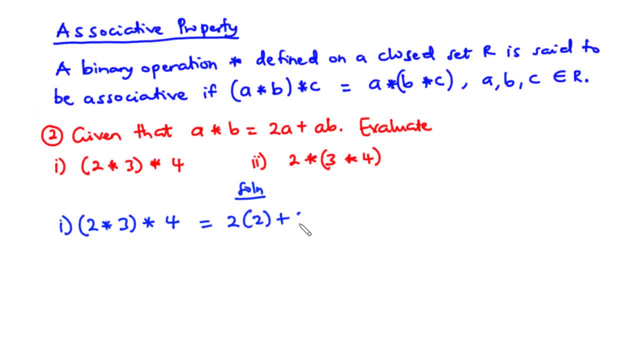 2 plus 2 times 3, all star 4. so 2 times 2 is 4, 2 times 3 is 6. 4 plus 6 is 10. so here we have 10 star 4. so we are going to apply the. 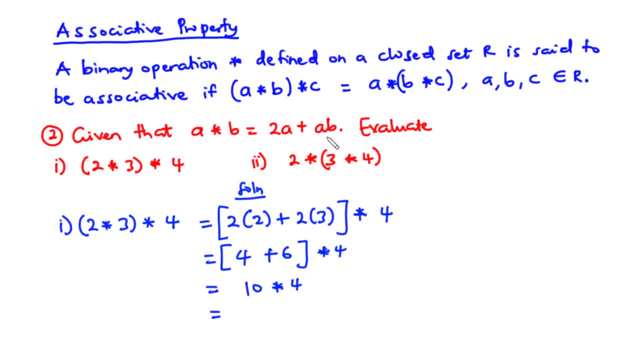 sequence: same rule: a star b equals to a plus a b. to solve: to solve a star 4. so this time a is 10, b is 4. so we have 2 times 10 plus 10 times 4. 2 times 10 is 20, 10 times 4 is 40, so we: 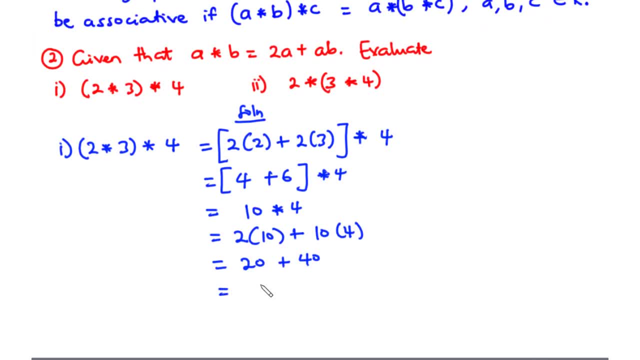 have 20 plus 40, which is 60 B, it's 20. in this case, hut b is 4. what is the b stick? take a couple of coins: 2 minus 2 times a b, so in both cases will be 20 b plus 2. 2 plus 2 times a. b plus 2 times a. b must be equal to 16. so that means 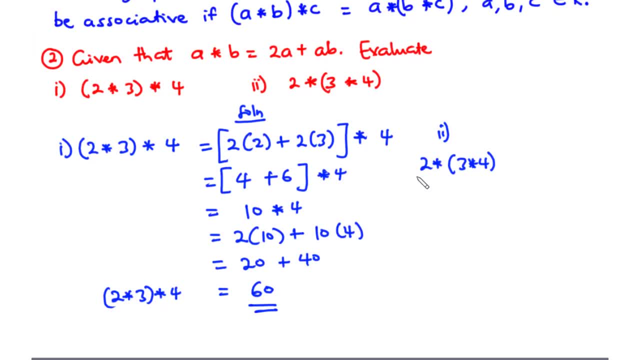 for this ask. first sheet in integral I she will present***. So let's take I, I So we can also solve for II. Lets solve for II, So for II in brackets. That is 2. star 4 is 9. wall became a phase 4 stars through 18. 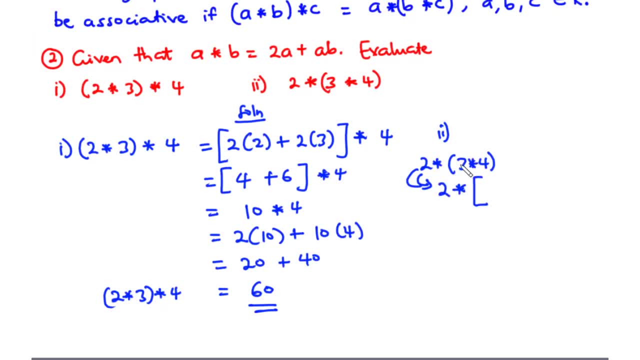 star in a bracket. This time our a is 3, our b is 4.. So, using this rule, we have 2 times a, which is 3, plus a, which is 3 times 4.. So that's going to be 2 star 2 times 3 is. 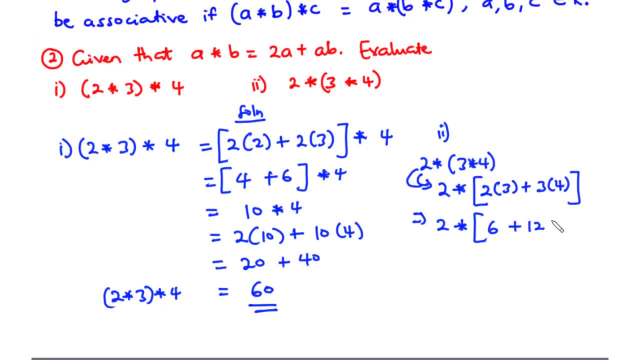 6.. 3 times 4 is 12.. 6 plus 12 is 18.. So this time we have 2 star 18.. So we are going to use the same rule to solve that. So a is 2, b becomes 18.. So that is 2 times 2 plus 2. 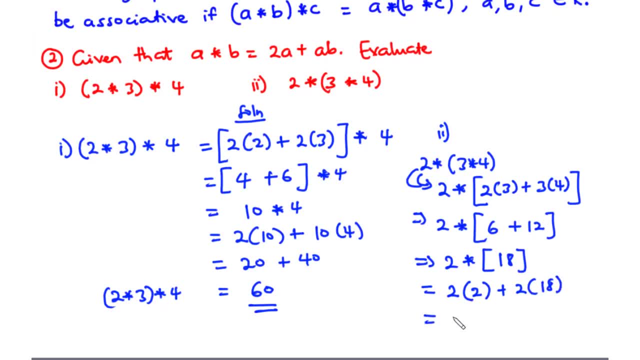 times 18.. 2 times 2 is 4.. 2 times 18 is 36.. So 4 plus 36 is 40. So 2 star into bracket 3 star 4 is equal to 40. Now because the two values or the two numbers are not the same, we say: 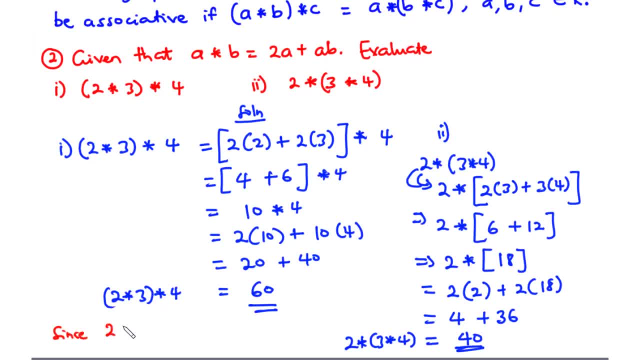 that since 2 star 3 in a bracket, star 4, is not equal to 2 star 3, star 4 in a bracket, then the binary operation star is not associative. So now let's move on to the distributive property. So for the distributive property. 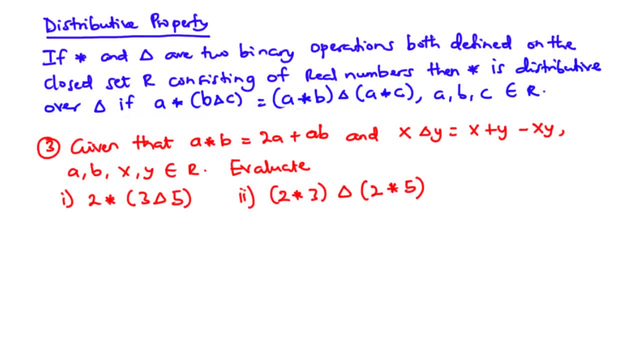 we are saying that if star and delta are two binary operations, both defined on the closed set R consisting of real numbers, then star is distributive over delta. if a star into bracket b, delta c is equal to into bracket a star b, delta into bracket a star c. So we 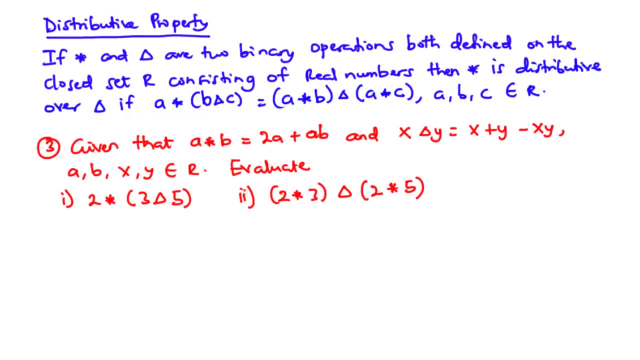 have two binary operations, star and delta. So we are going to check whether a star into bracket b, delta c is equal to into bracket a star b, delta into bracket a star c. Now if the left hand side is equal to the right hand side, we say that star is distributive. 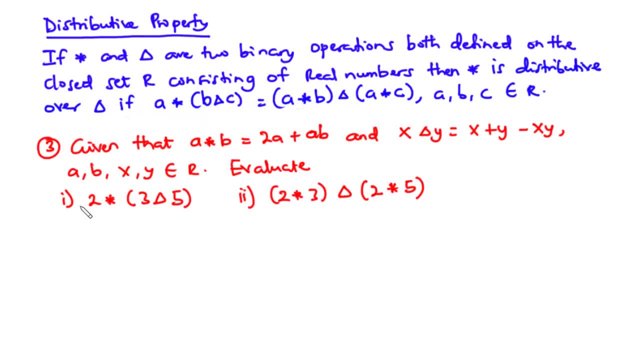 over delta. So let's do that by solving this question. Given that a star b is equal to 2a plus ab and x delta y is equal to x plus y minus xy, where a, b, x and y are all members of the. 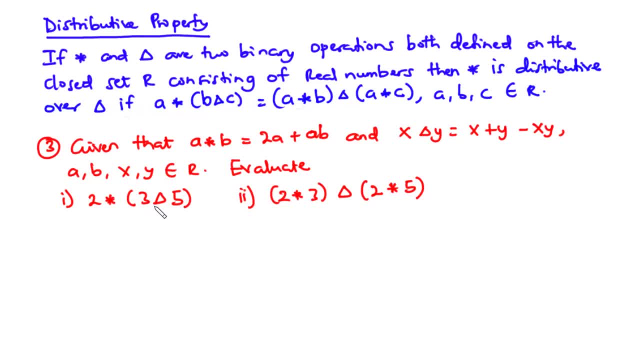 set R. we are going to evaluate 2 star into bracket 3 delta 5, and then ii, 2 star 3 in a bracket delta 2 star 5.. So we are going to combine what's in the bracket first, that is, 3 delta 5.. So this is equal. 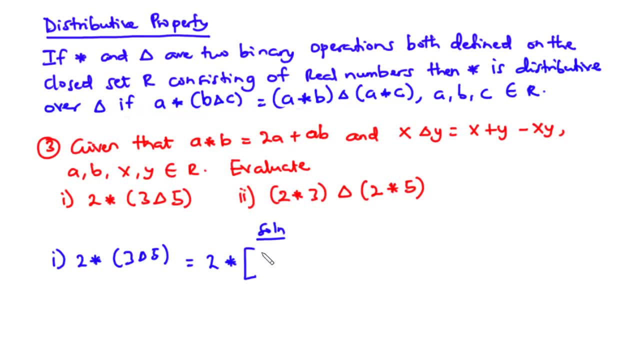 to 2 star into bracket. we are going to apply x delta y to this binary operation, So x is 3, y is 5.. So we have 3 plus 5 minus 3 times 5.. 3 plus 5 is 8, 3 times 5 is 15.. 8 minus. 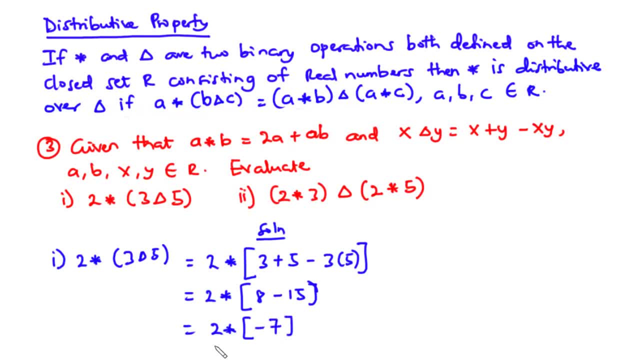 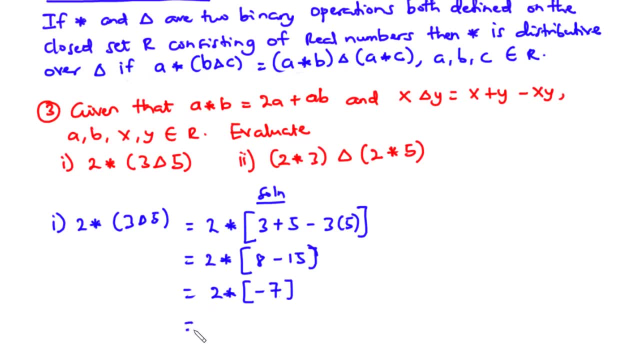 15 is negative 7.. So now we have 2 star negative 7.. So we are going to use the operation star to combine 2 and negative 7.. So, using this, we have 2 times a. Now our a is 2, our b is negative 7.. 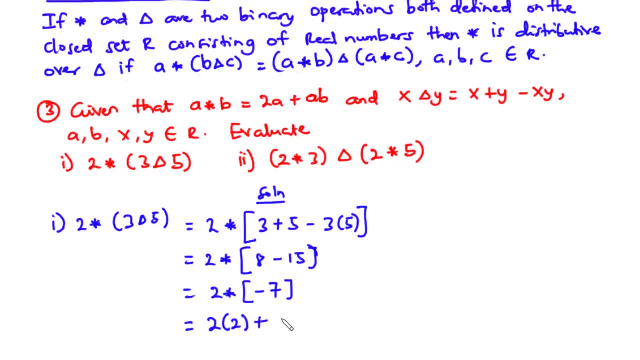 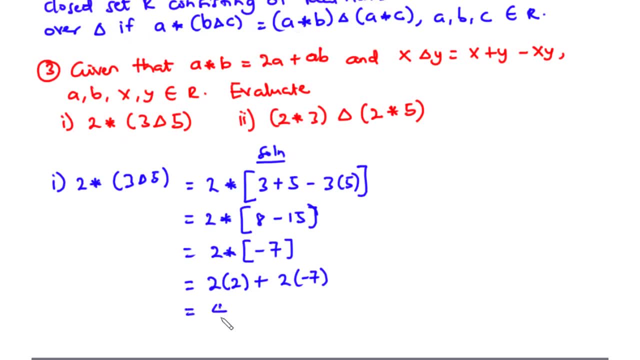 So 2 times 2 plus 2 times negative 7.. 2 times 2 is 4.. 2 times negative, 7 is negative 14.. And then 4 minus 14 is equal to negative 10.. So 2 star into bracket 3 delta 5 is equal to negative 10.. 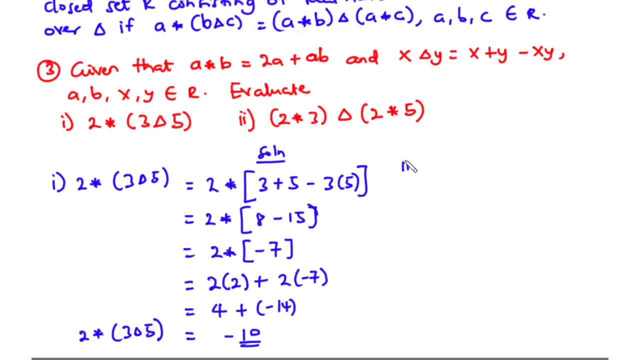 Now let's solve for ii. Here we have 2 star, 3 delta, 2 star, 5.. So we are going to apply the binary operation star on 2 and 3.. So, using this rule, 2 times 2.. 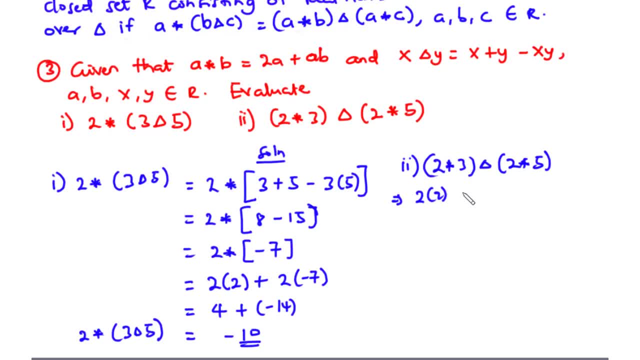 Now our a is 2 and then our b is 3.. So 2 times 2 plus 2 times 3.. All in the bracket delta Here. our a is 2, our b is 5.. So we have 2 times 2 plus 2 times 5.. 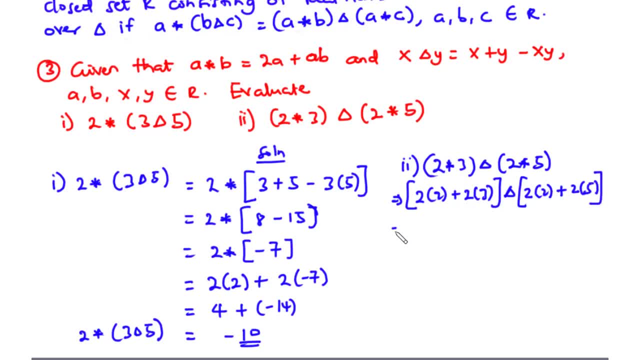 So 2 times 2 is 4.. 2 times 3 is 6.. 2 times 2 is 4.. 2 times 5 is 10.. 4 plus 6 is 10.. So we have 10 delta. 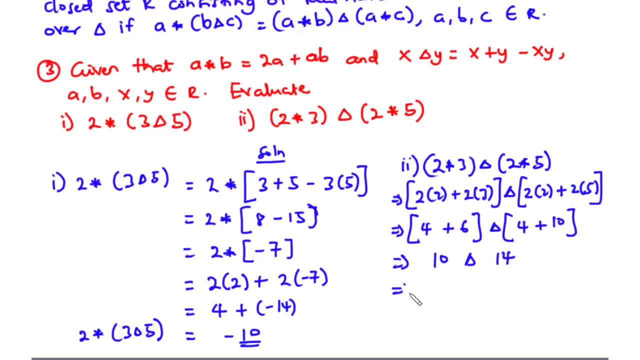 4 plus 10 is 14.. Now we have 10 delta 14.. So we are going to apply the binary operation: delta On 10 and then 14.. So we are going to use this. So x is 10, y is 14.. 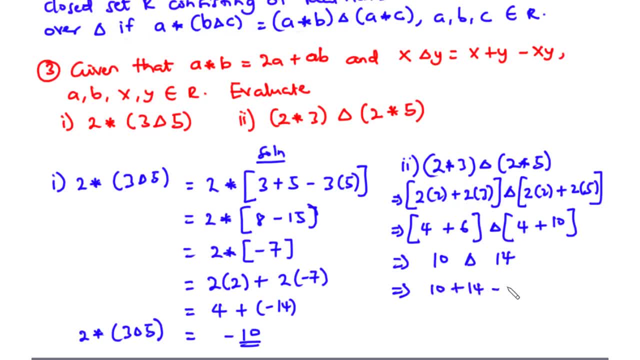 So we have 10 plus 14 minus 10 times 14.. 10 plus 14 is 24.. 24 minus 140 is negative 116.. So we have 2 star into bracket 3, delta 5 to be negative 10.. 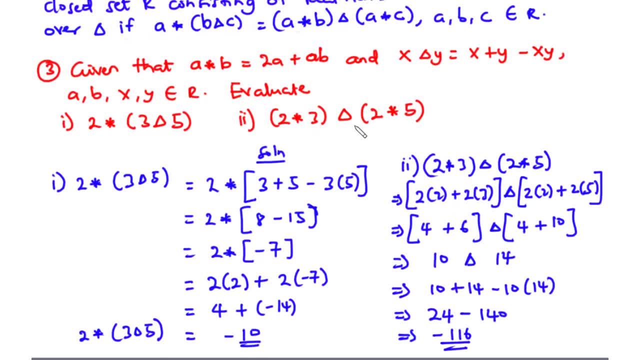 And then 2 star 3 delta 2 star 5 as negative 116.. So since 2 star into bracket 3 delta 5 is not equal to 2 star 3 delta 2 star 5, it follows that star is not distributive over delta. 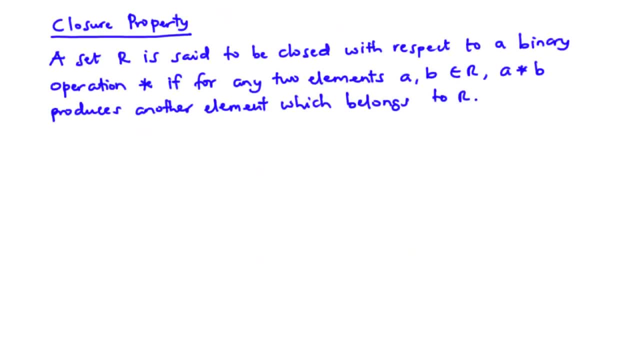 So the binary operation of the set R is closed, So we have the set R in place. So, lastly, let's talk about the closure property. Now we are saying that a set R is set to be closed with respect to a binary operation star. 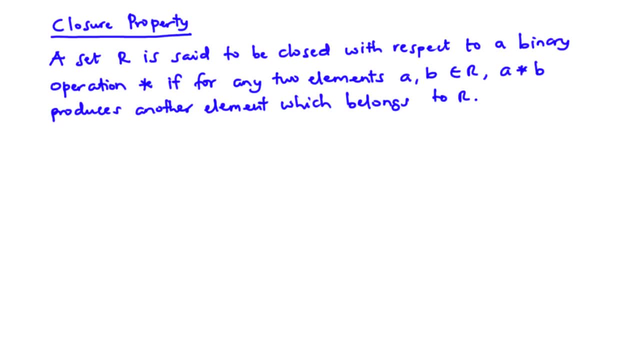 If, for any two elements, A and B, which are members of the set R, A star B produces another element which belongs to the set R. So for instance, let's say we have a set R. Let's say we have a set R.